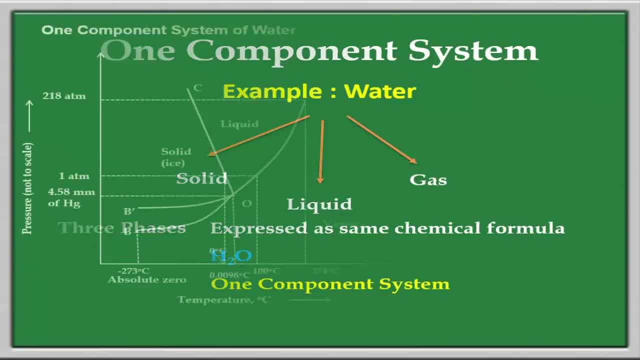 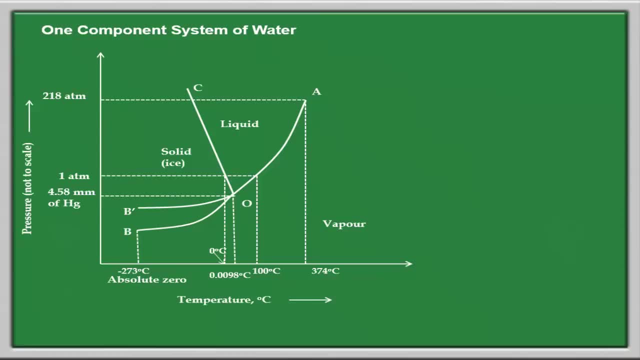 component system. Let us see the phase diagram for the system of water. As we can see, the temperature is on the x-axis and the pressure is on the y-axis. The phase diagram consists of three curves: curve OA, curve OB and curve OC. There are three areas: area AOB, which consists of vapor phase. 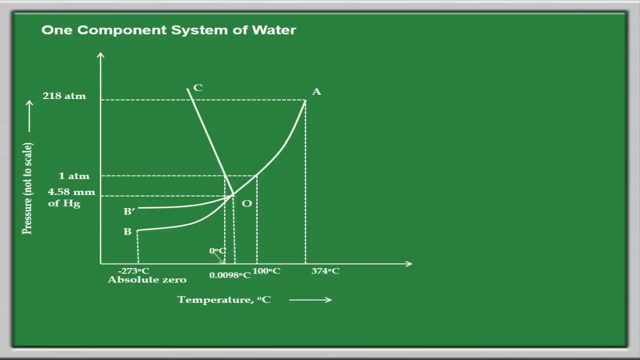 area AOC, which consists of liquid phase, and area BOC, which consists of solid phase. All these three curves meet at the single point O, which is called as triple point of water. We study phase diagram because phase diagram is a one component system. It is a one component system, It is a one component. 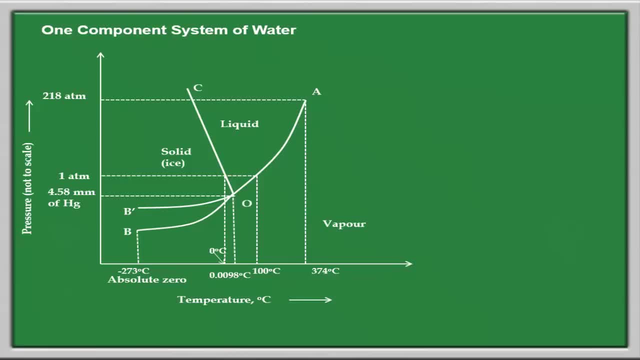 system. The phase diagram allows us to understand in what state matter exists under certain conditions. Now let us understand this phase diagram. First, we will study the curves. We will start from the curve OA. The curve OA starts at point O, which is triple point of water, and ends 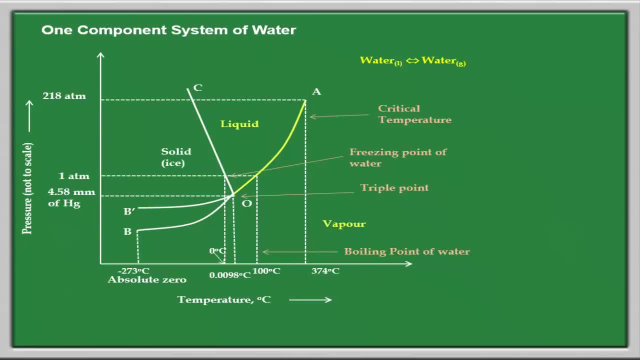 at point A, which is called as critical temperature. Above critical temperature there is negligible amount of water which is in the liquid state. Along this curve, OA, liquid and vapor phase are in equilibrium. Therefore this curve is called as vapor pressure curve. In the curve OB it starts. 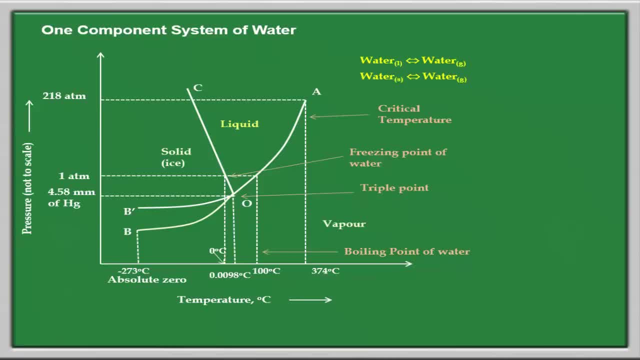 at point O and ends at point B, which is absolute zero. Along this curve, solid phase and vapor phase are in equilibrium. Therefore this curve is called as sublimation curve. The third curve, that is curve OC, starts at point O, ends at point C, and along this curve, solid and liquid phase are in equilibrium. 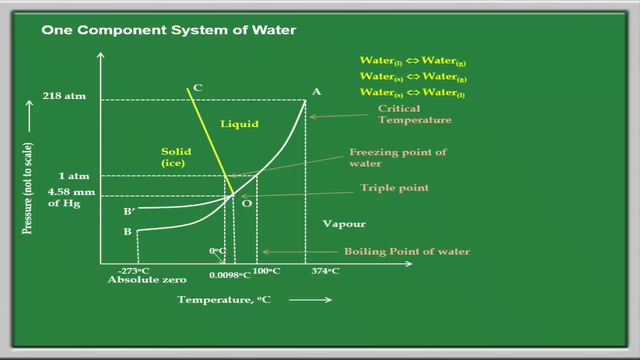 Therefore this curve is called as melting point curve Or fusion curve of ice. The inclination of the curve OC towards the pressure axis indicates that the melting point of ice is lowered by increase in pressure. So if we observe any curve, there are two phases are in equilibrium. Therefore, when we apply the phase rule, that is, F is equal to C minus. 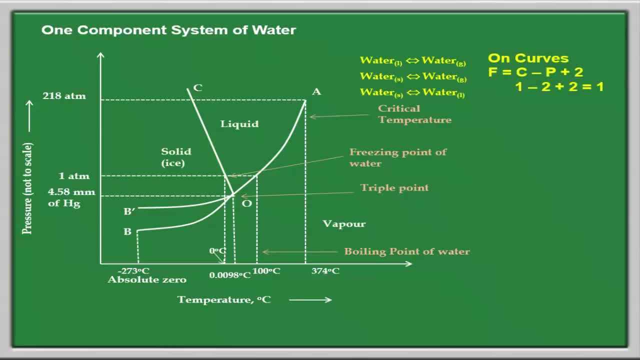 P plus 2, where F is degree of freedom, C is number of components, P is number of phases. So we are studying system of water and we have already seen that the number of component is 1.. And in case of curves, there are two phases which are in equilibrium. Thus the number of phases are 2.. 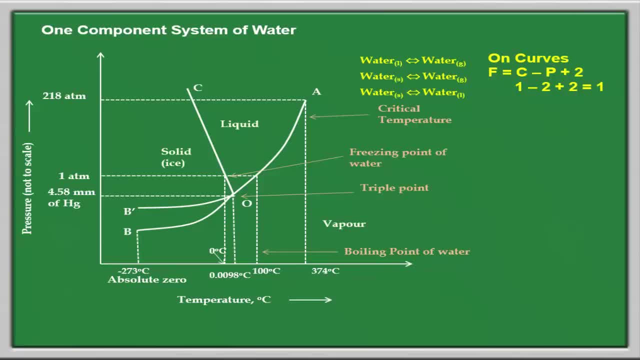 So 1 minus 2 plus 2 is equal to 1.. So all the curves are univariant. That means if you select a particular temperature, the pressure is automatically fixed, and if you select a particular pressure, the temperature is fixed. So to decide any point on the curve you require any one variant, that is. 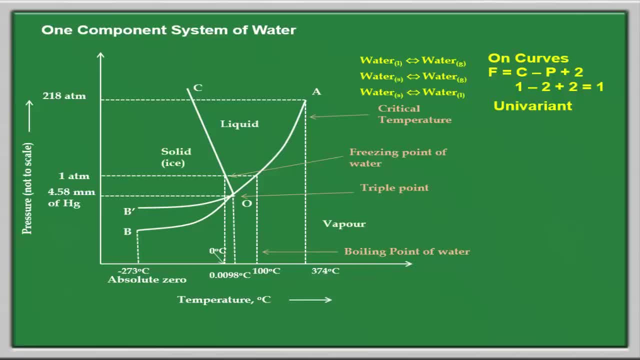 temperature or pressure. So we have two areas: In area AOC only liquid phase exist, In the area AOB only vapour phase exist And in the area BOC only solid phase exist, That is, the ice exist In any particular area there. 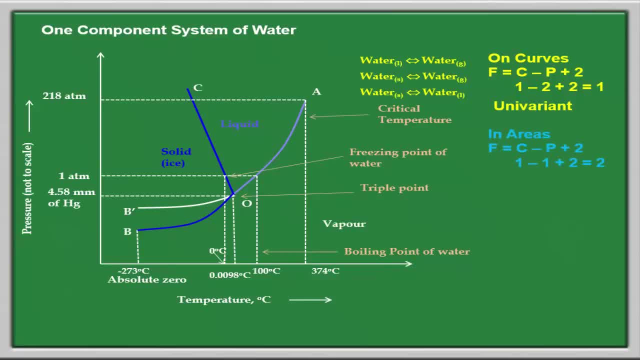 exist only one phase, So number of component is 1.. Number of phase is also 1.. So 1 minus 1 plus 2 is equal to 2.. That means you require two variants to fix any particular point or to understand any particular state in the particular area. Therefore, all the areas are bivariant. 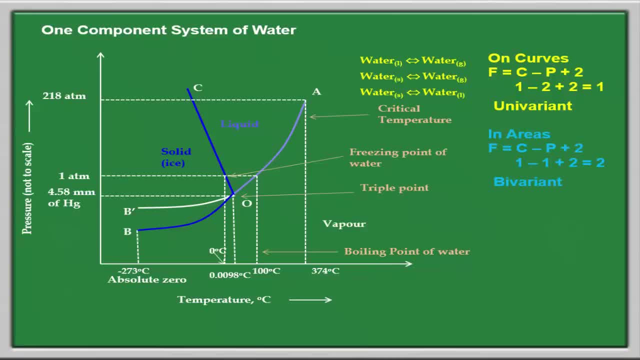 All these three curves meet at the single point, O, which is called as triple point of water, That is, ice is in equilibrium with water, which is in equilibrium with water vapour. So if we apply the phase rule, F is equal to C minus P plus 2. Component is 1.. Phases are 3.. 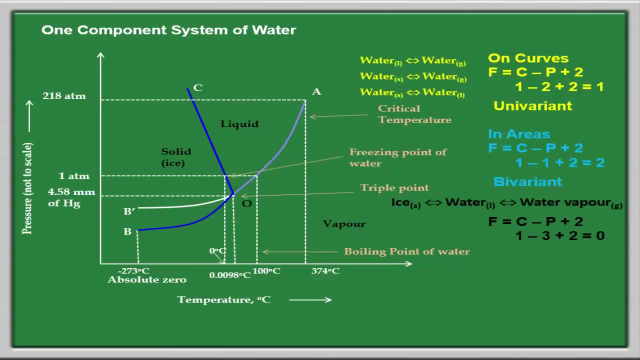 So F is equal to 0.. That means such system is possible Only at specific temperature and specific pressure, So it is a zero variant. The specific temperature is 0.0098 degree Celsius and the pressure is 4.58 millimeter of mercury. 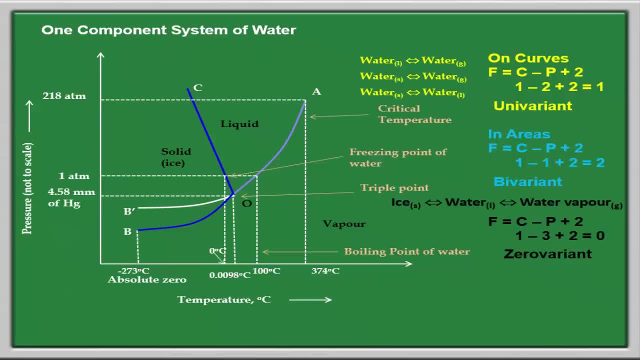 In addition to this, we can see one additional curve curve OB dash, which is called as metastable state. It states that it is possible to super cool the liquid water below 0 degree Celsius, keeping it in the liquid state. That means water can be kept in the liquid state. That means water can be kept in the liquid state. 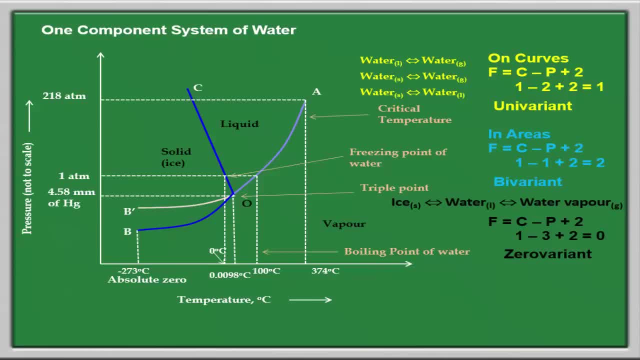 Below 0 degree Celsius, provided there is no impurity present in water. So this is called as super cool water. but any disturbance from the temperature or pressure or if any impurity is present, the whole liquid will turn into a solid. This is because the curve OB dash is above curve OB, which is in the solid area.